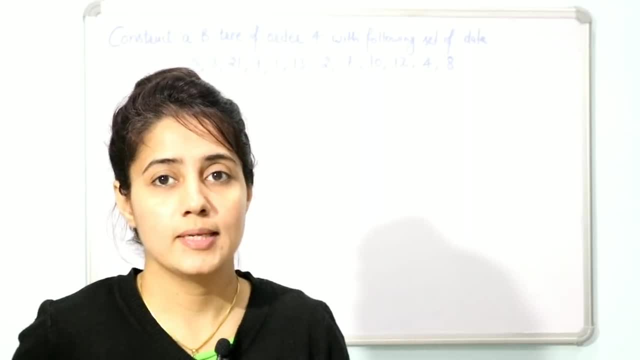 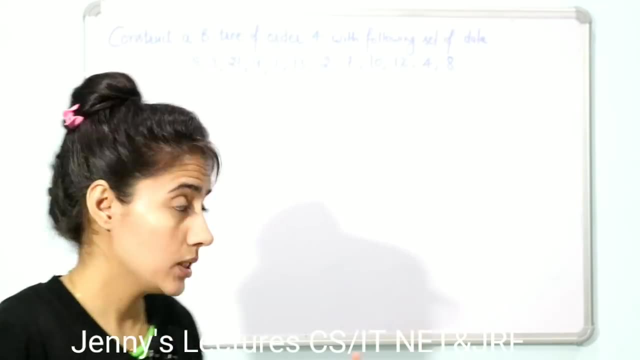 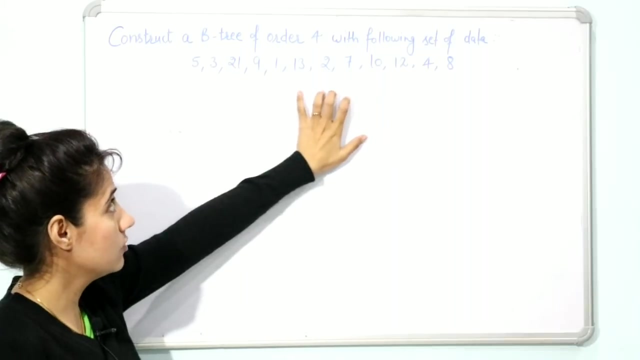 Hi guys, welcome back to my channel, and in this video I am going to discuss with you how to construct a B tree of order 4.. So the question is: construct a B tree of order 4 with the following set of data: We are given some integers and we are supposed to create: 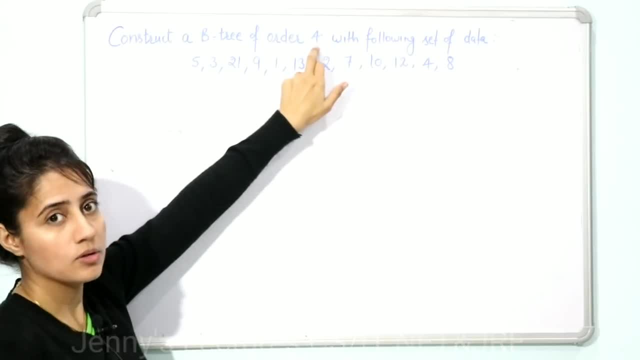 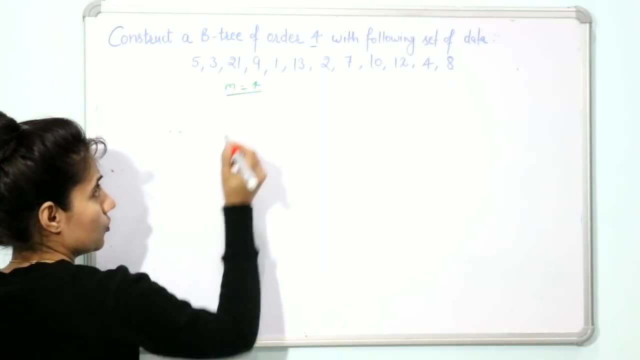 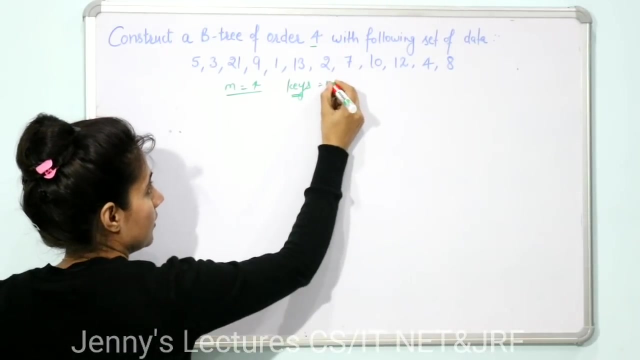 a B tree and that B tree will be having order of 4.. See, the order is 4 means m value is 4.. So maximum keys any node can have is m minus 1, that is 4 minus 1 and that is 3.. Now 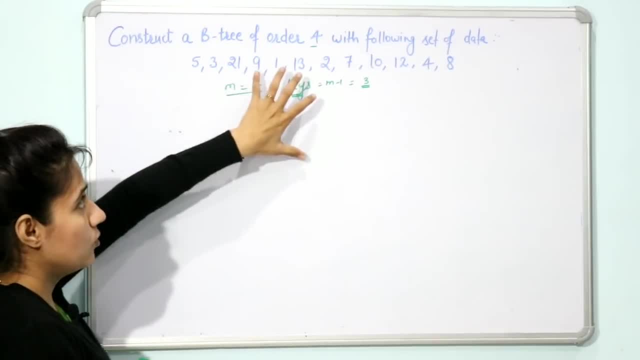 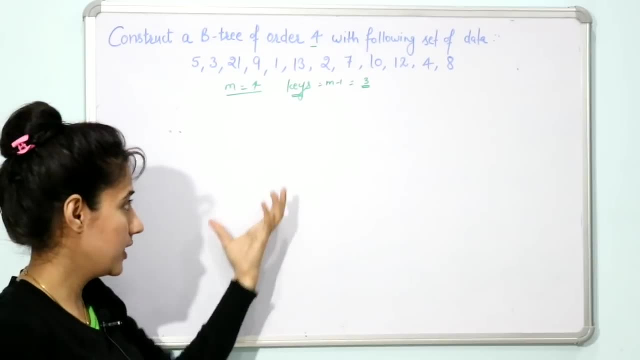 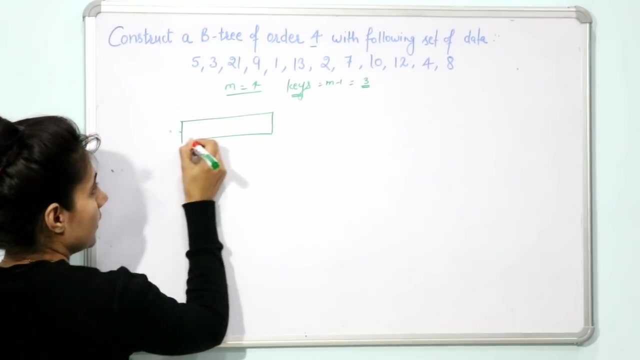 see. first of all, scan this given set of data from left to right. First number is 5.. We will insert this 5 into B tree, but initially we have empty B tree, So one node will be created. One node will be created and that node can have maximum keys 3.. Okay, 1, 2 and 3.. First, 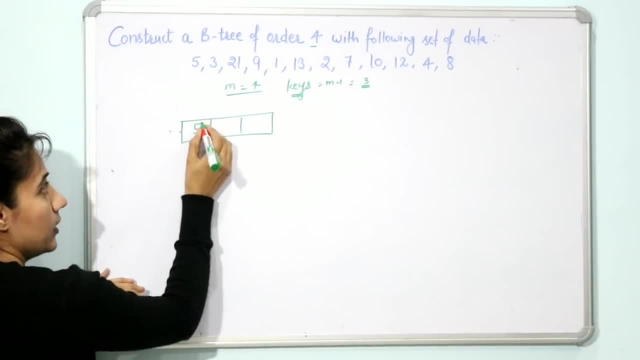 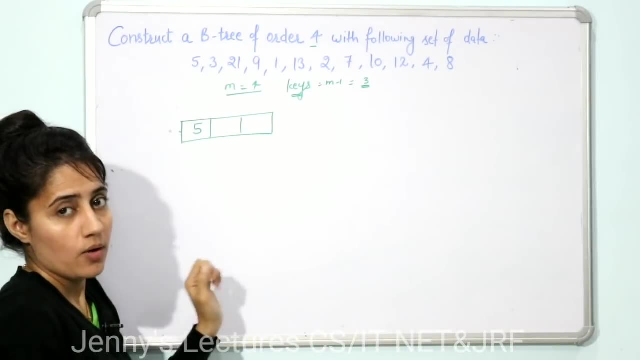 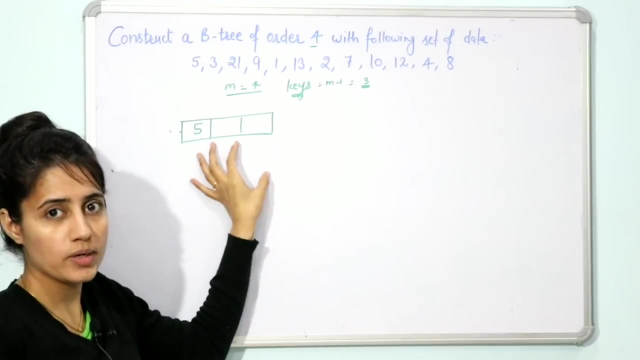 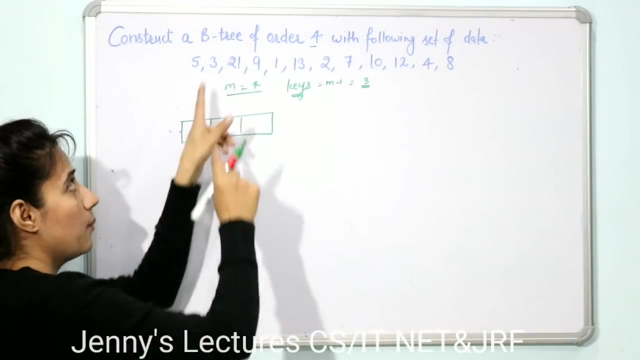 is first. number is 5.. 5 will be inserted at this position and this node Now. next is 3.. See, now, I have already told you that all the numbers in that node will be, you know, stored in ascending order, Or the data would be sorted fashion. So next number is 3.. We cannot put 3 at this place. 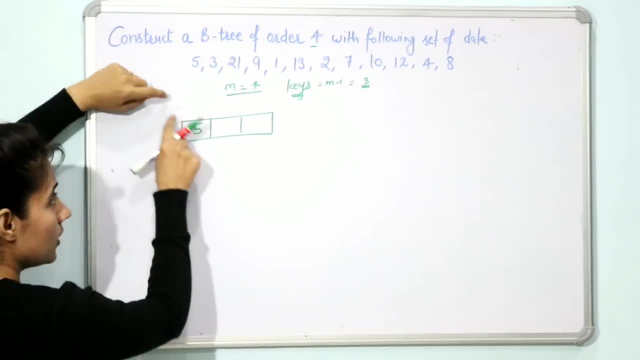 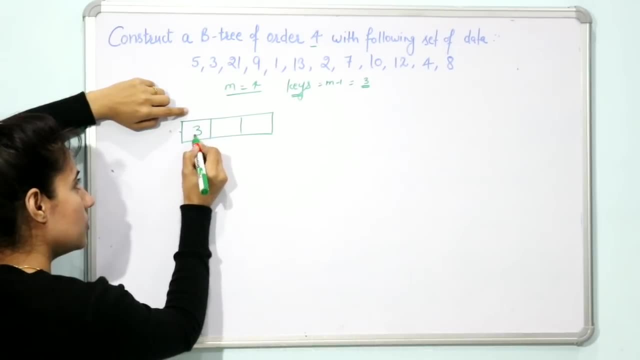 Why? because 3 is less than 5.. So first of all we will compare 3 with this one. 3 is less than 5.. Okay, so where 3 will inserted 3, and here it will be 5.. Fine, next is 21.. 21 would be inserted at this place. So 21 is the number, See 2 and 3 are the numbers. All that is 3.. So next 3 would be inserted at this place. So next number is 3.. Next this: 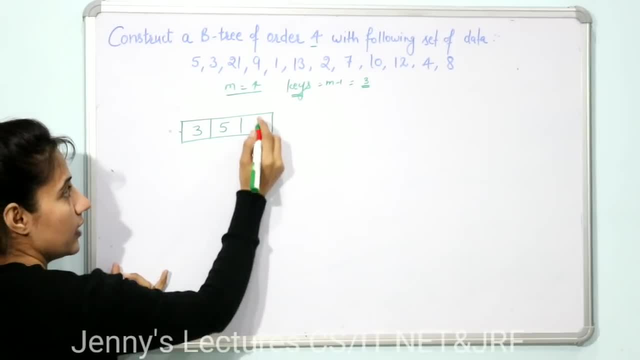 one is 5.. So next 3 will be inserted, 3, and here it will be 5.. Next is 21.. 21 would be inserted, which place greater than 3, greater than 5, 21 is greater than 3 and 5 to 21 will. 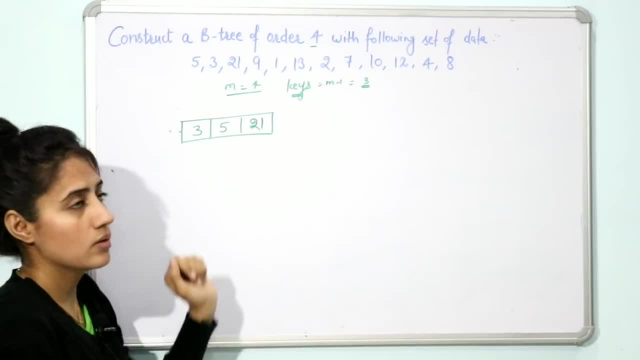 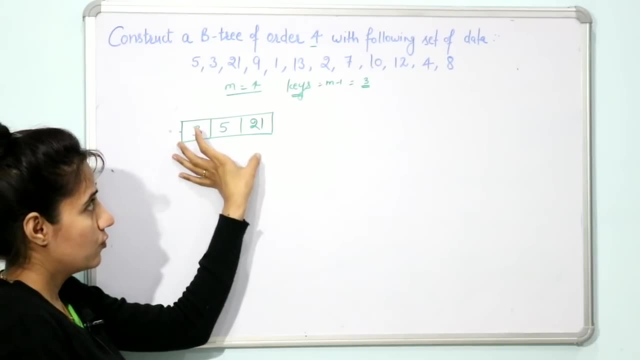 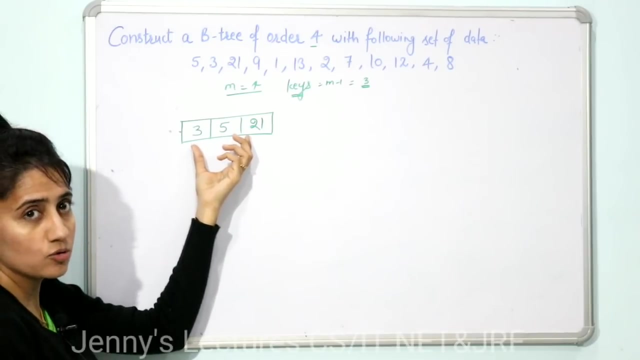 be inserted at this place now. next is 9. now, first of all. see, it's not like this node is full, because maximum we can insert only three keys, any- in any node. so firstly we would split this node and then we will insert this. 9, no, first of. 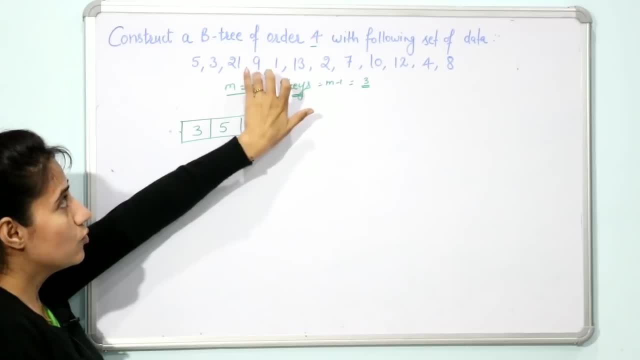 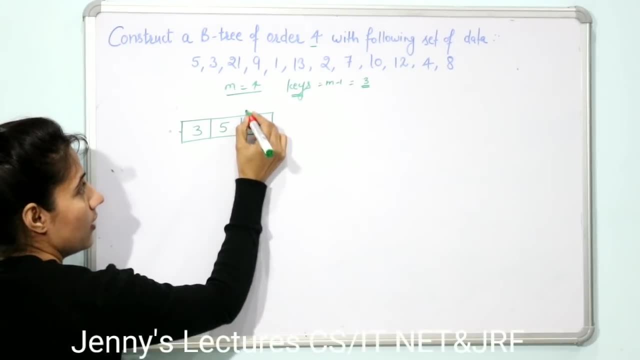 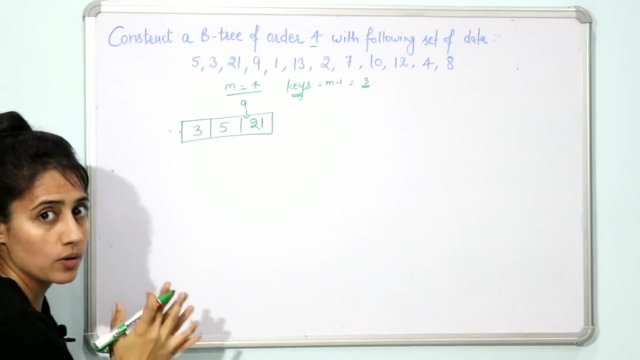 all. we have to find out proper place to insert this 9 in this node, where you can insert this 9 after 5, means at this place before 21 and after 9, 3, 5, after 5, 3, 5, 9 and 21. now now see, maximum keys can be 3 only and, but in this node we. 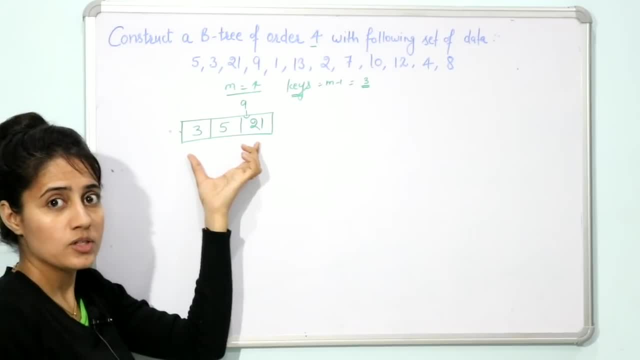 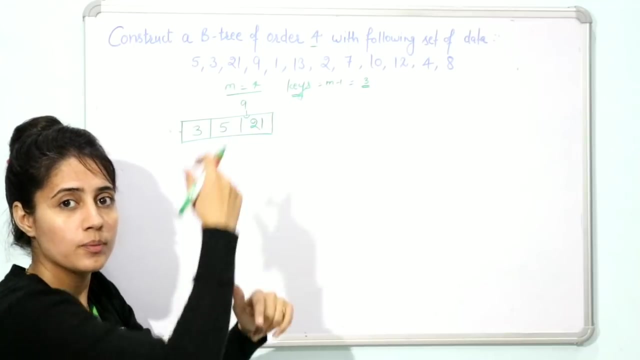 have 4 keys. so what is the procedure now? this tree would be splitted in two parts. how this splitting will be done, we'll find out the median, or you can see the middle element of this node and that middle element would go one level up. or you can say to the parent of this node: but obviously you can see in this node. 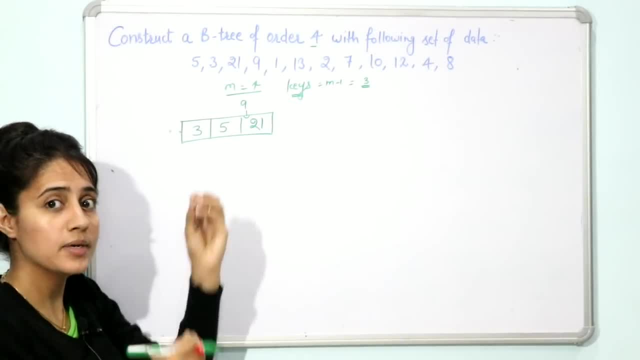 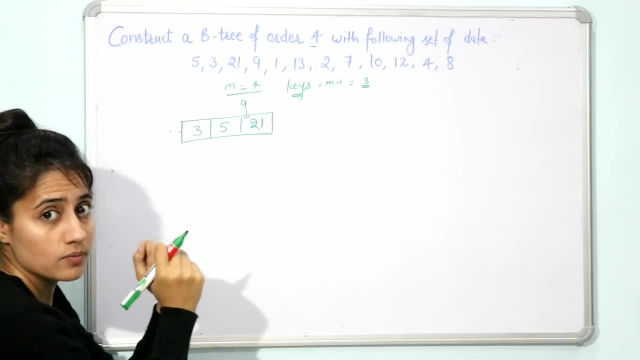 we have only one node, root node, so parent is no one. in that case, that middle element would go one level up and that middle element will become the root. and what will happen to 2 of this root? children now see 3, 5, 9 and. 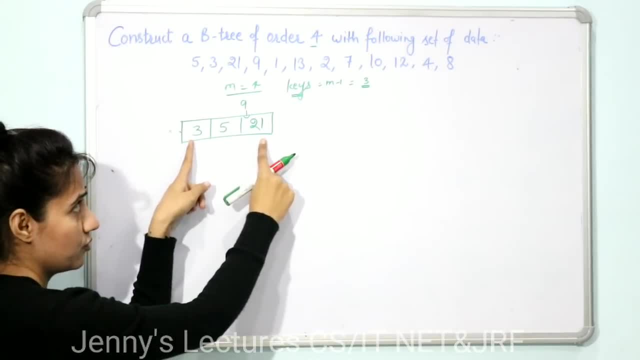 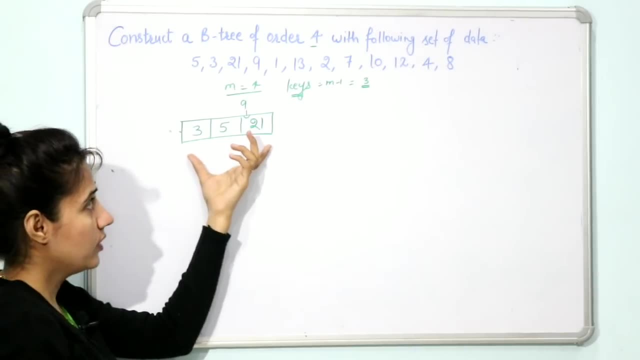 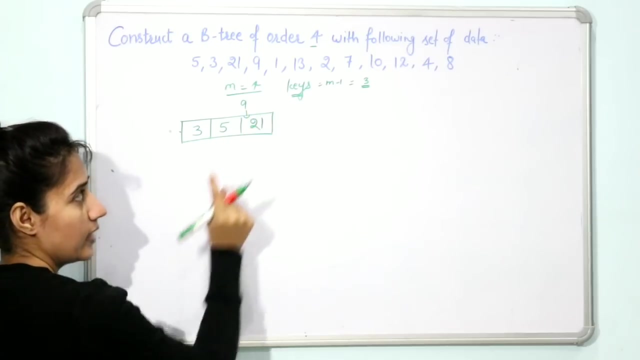 21. now what is the middle element of this one? we have only four numbers now the middle element can be: see, you are even number here to middle element is kiddo. so then 5. either you can take 5 as a middle element or you can take 9 as a. 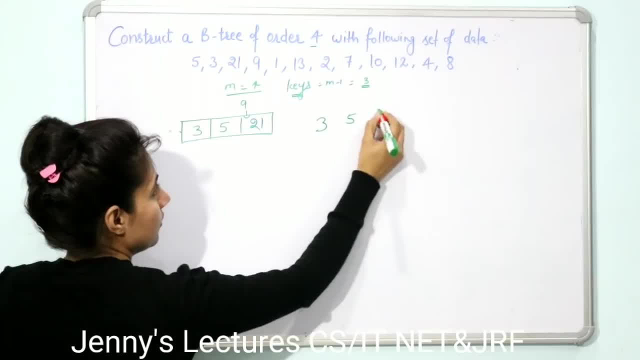 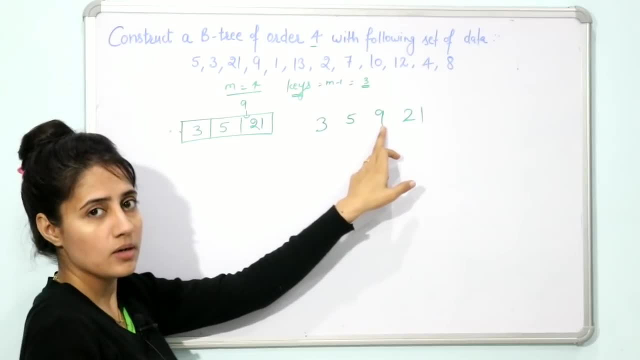 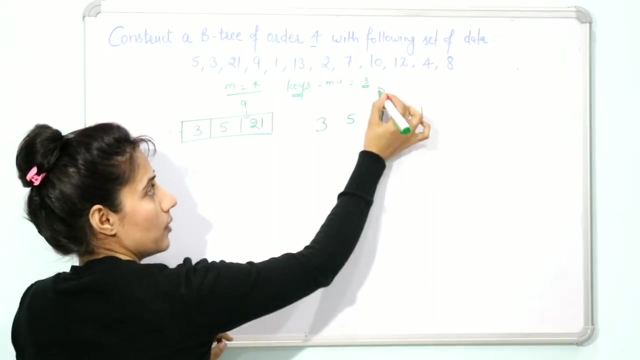 middle element: 3, 5, 9 and 21. sorry, either you can take 5 as a middle element or 9 as a middle element. if you take 5 as a middle element, then the tree up create Kuroki book, yoga, 5, popco per chalaja, and the left child of 5 is 3, the right child of 5 is 9 and 21. 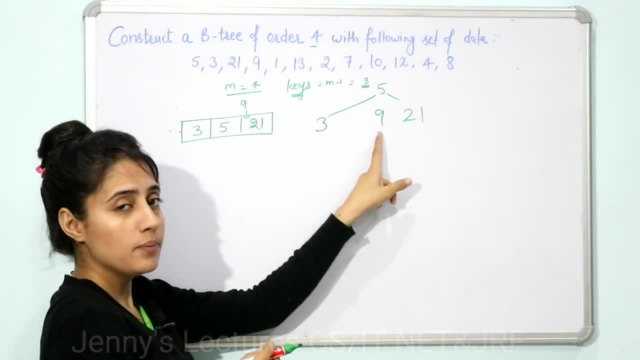 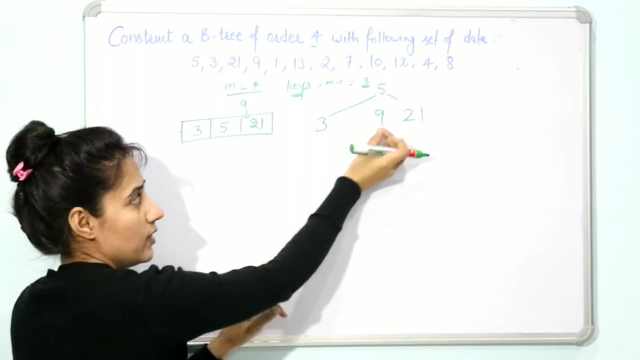 okay, if you take 9 as middle element, then what will happen? 9 would go one level up, 9. here again, the left side of 9 would be 3, 5 and right would be 21, and this one: 3, 5 and right would be 21. 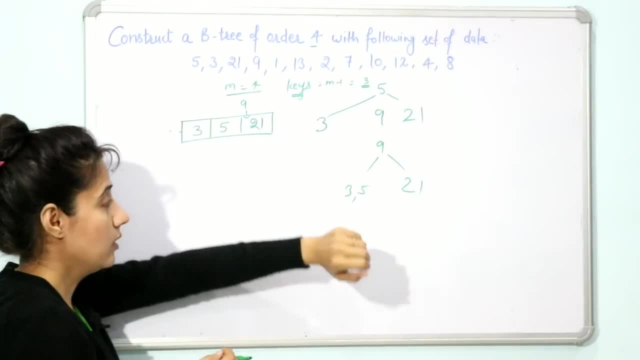 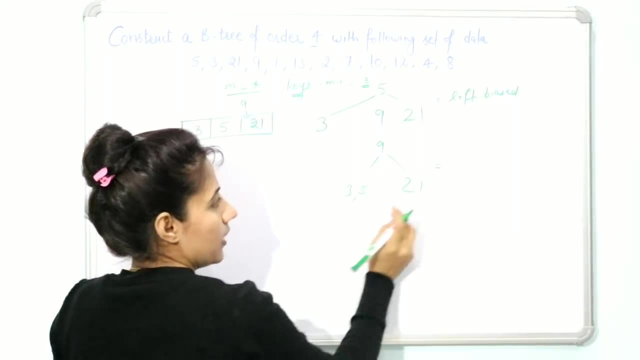 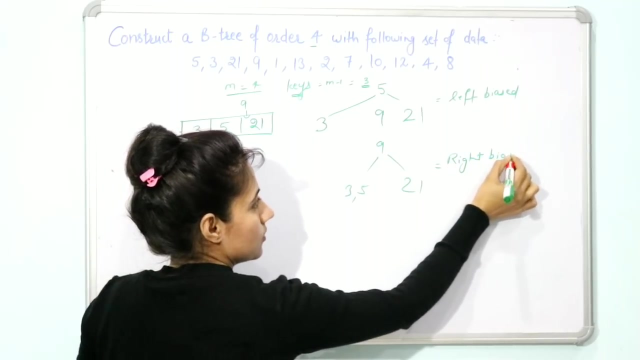 okay, both trees are right now. this tree is known as left biased and this tree other app I see, create Kuroki. if you would create, take 9 as middle element and this is known as right biased. a poebis miss a middle element. Lisa to. 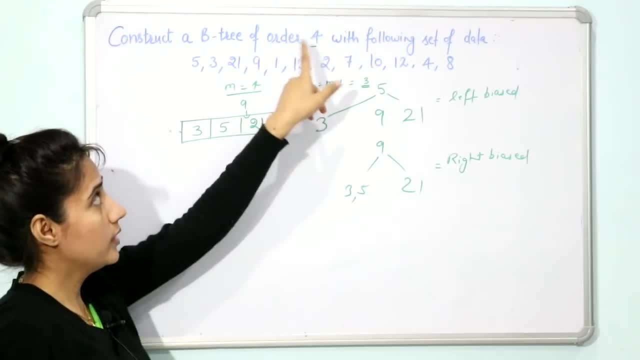 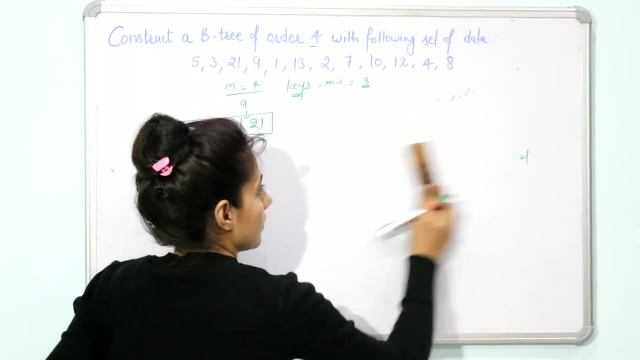 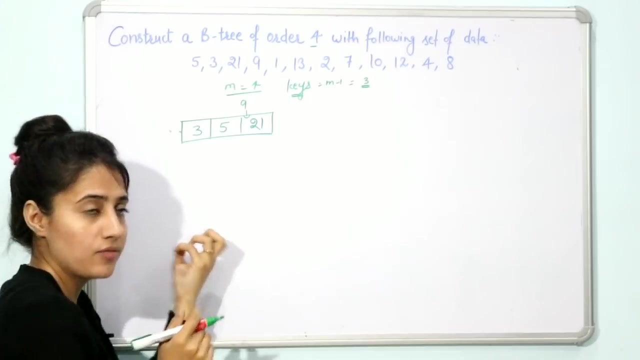 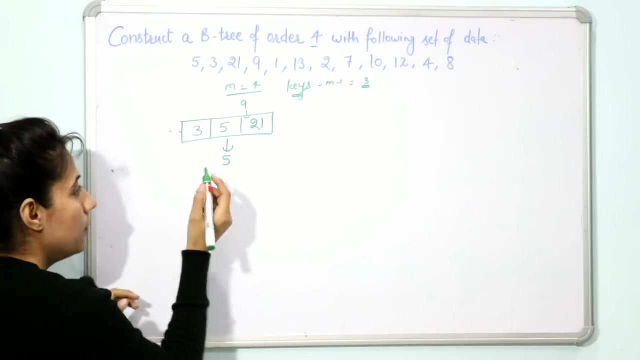 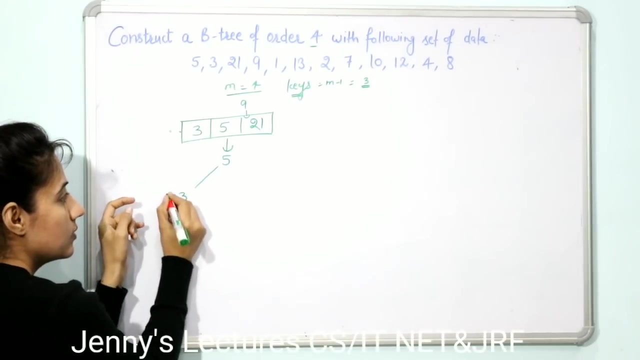 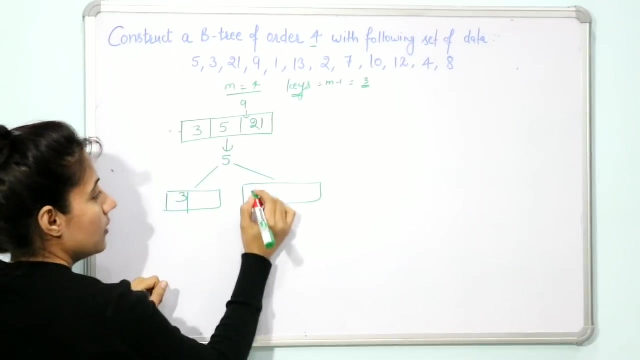 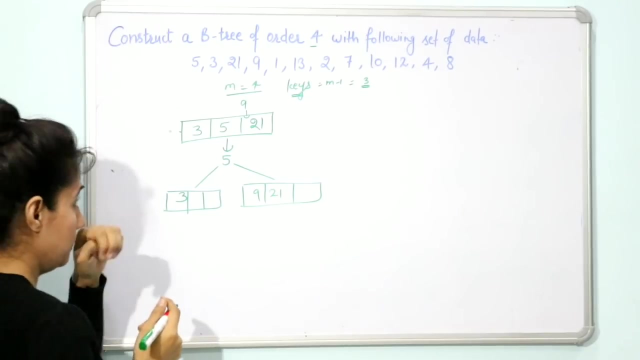 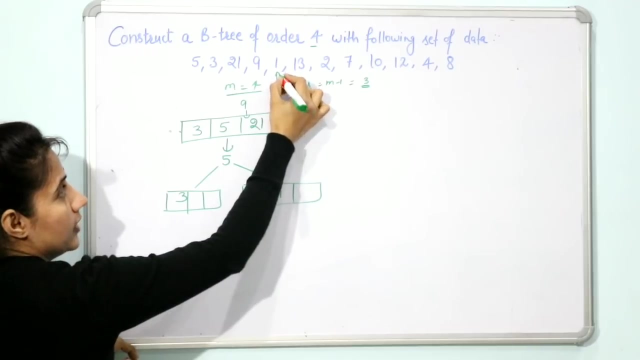 take it when you know the order is. even in that case, it will happen, so you can start fromí. OK, and the right would be Kurok, episode 11, 9 and 21.. Fine, Okay, Sorry, The next number is 1.. 9, I have inserted. The next is 1. Now 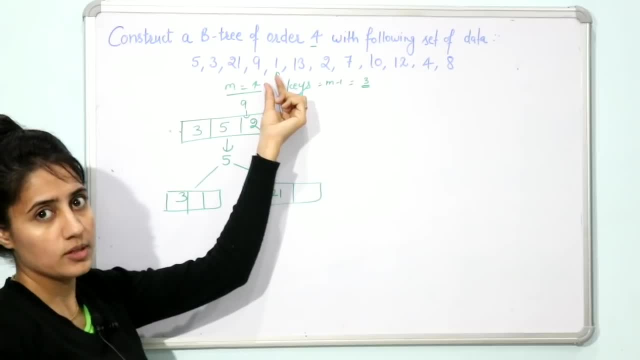 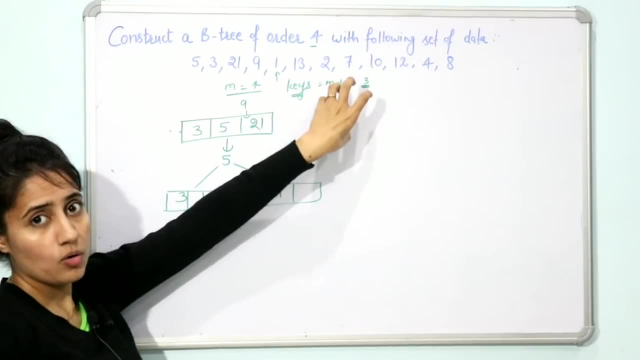 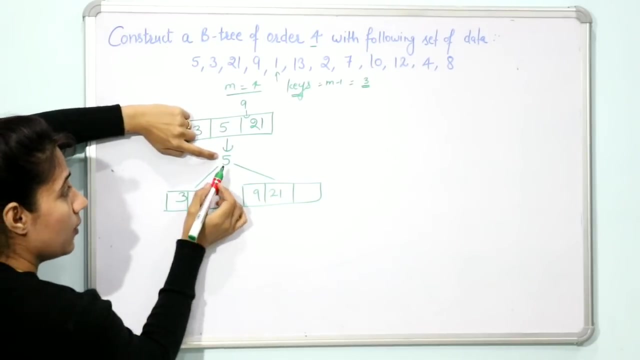 you have to find out the proper position to insert this 1 in this B tree And one rule is that any new number will always be inserted in leaf node. You cannot insert into root node 1.. But firstly we will compare this: 1. What will always be compared when we insert? 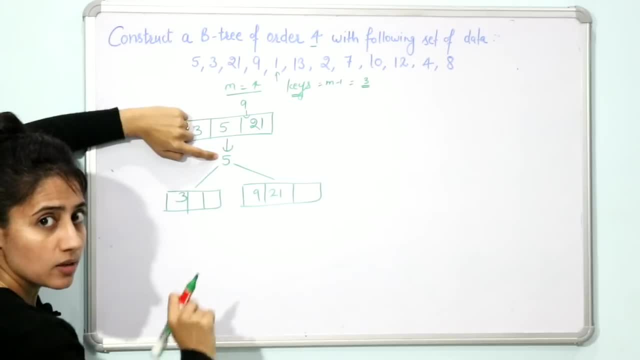 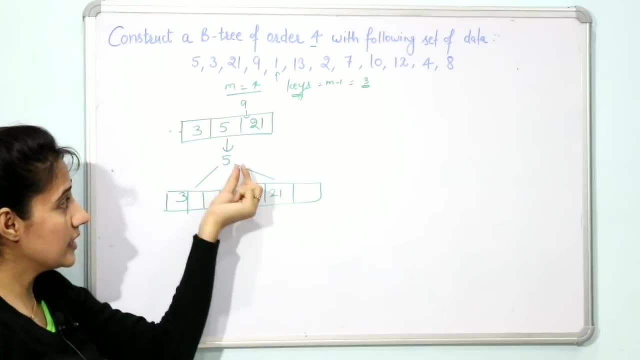 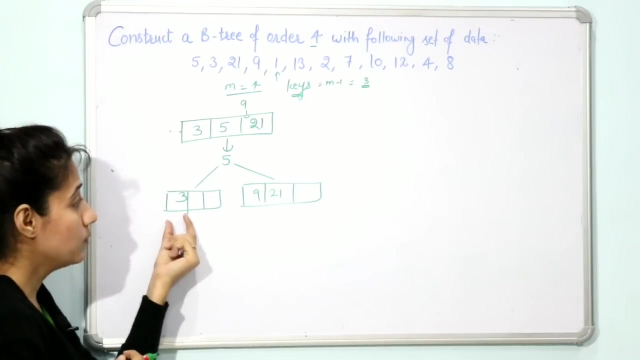 from the root node. Compare will start from root node but insert will always be in leaf node, So 1 would be compared with this 5.. We know 1 is less than 5. So we will go to the left part of 5.. Now we have 3 in this node. Now this is leaf node, So 1 would be. 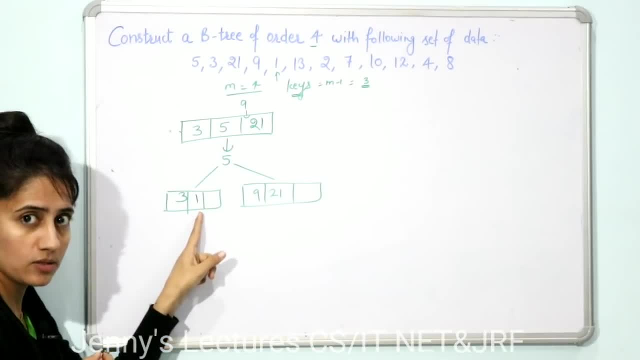 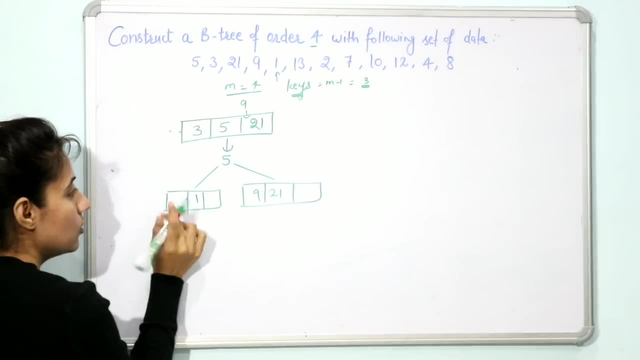 inserted at this place. But you cannot insert 1 at this place. Why So? because 1 is less than 3.. So it will be inserted in 3's left. So where will 1 be inserted At this place? and here would be 3.. Now, next is 13.. If we compare 13,, 13 is greater than 5.. We will 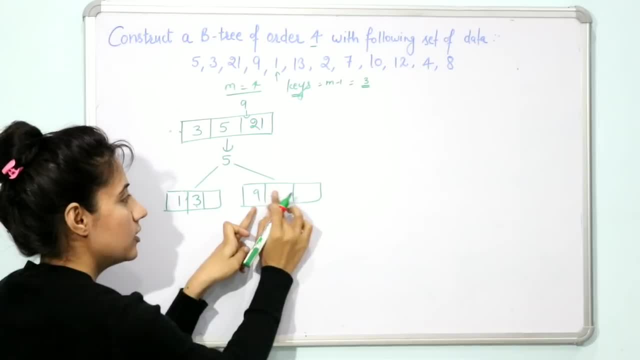 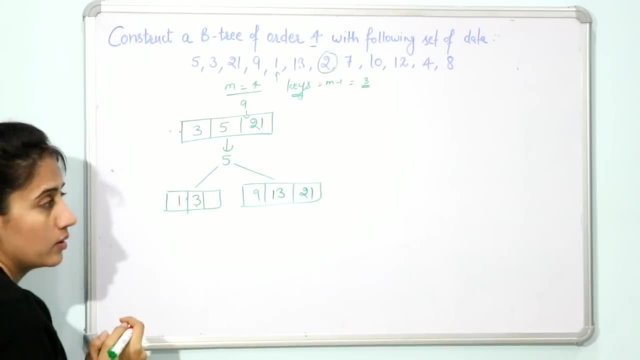 say, 13 is greater than 9 but less than 21.. So 13 would be inserted at this place 13 and 21.. Now, next is 2.. Now find out proper place for 2.. 2 is less than 5.. We will go. 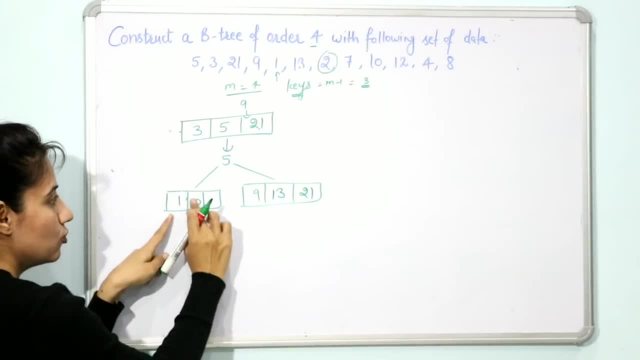 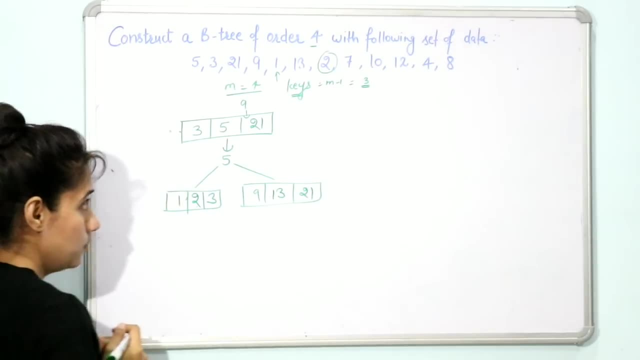 here 2 is greater than 1 and less than 3.. So 2 would be inserted at this place, 2 and 3.. Fine. Next number is 7.. Now find out: 7 is greater than 5.. So we will go to the right. 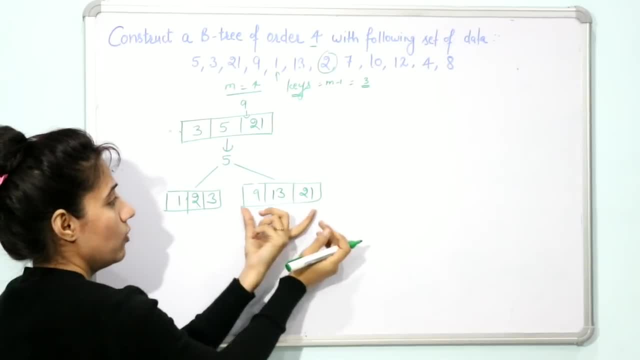 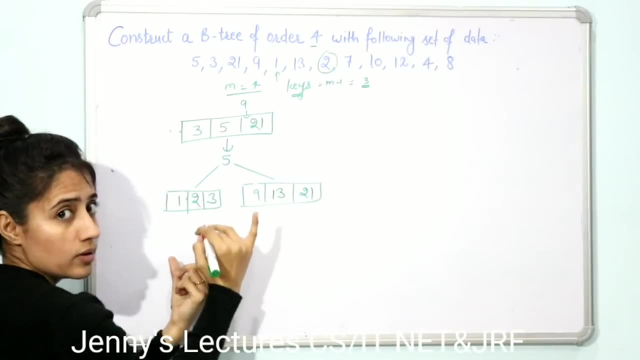 part Greater than So. if it is less than, then we will go to left. Now find out the proper place for 7. After that, we will split this node. Now 7 can be inserted at this place Before 9, Because 7 is less than 9, less than 13 and less than 21, obviously. 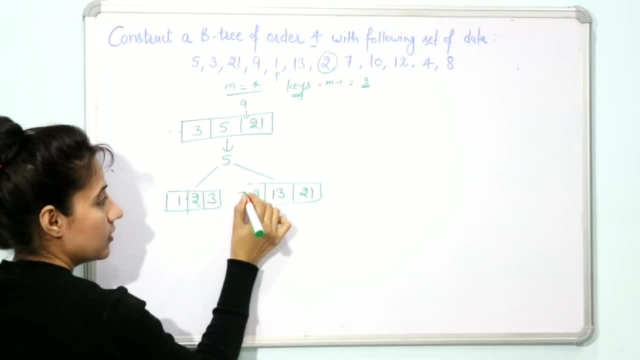 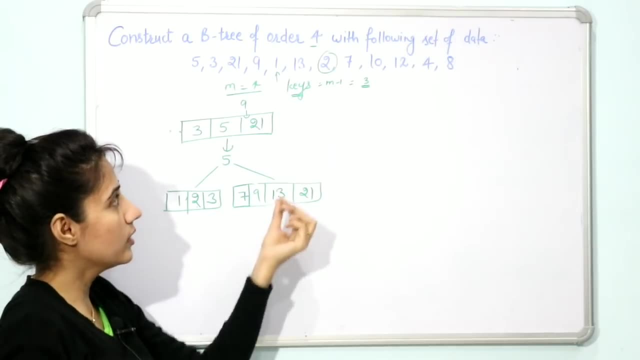 So where should 7 be inserted At this place? 7, But we cannot insert 7 at this place. Why so? Because maximum key any node can hold is 3 only, So splitting would be done. Now how will you do splitting? It is the same. 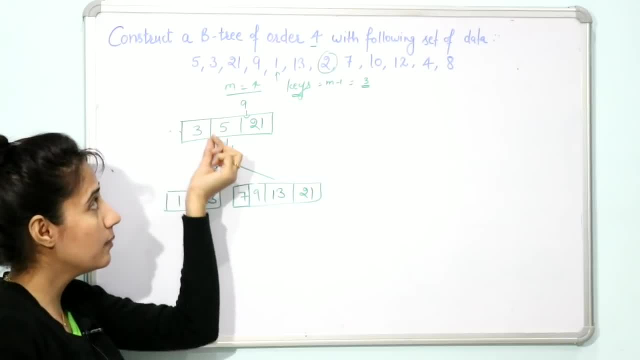 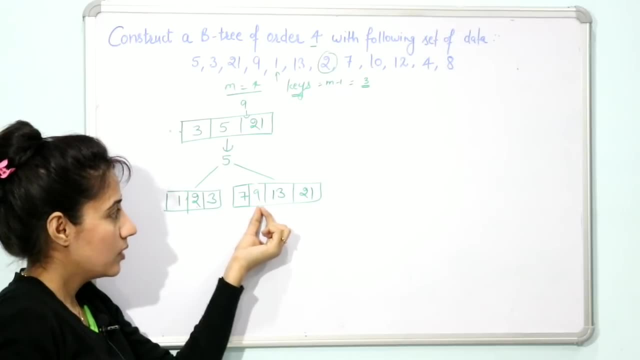 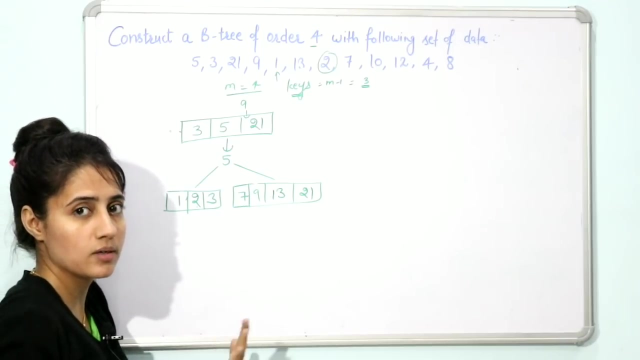 You have to find out middle element. Now here we had taken middle element 5, Means tree was left biased. Ok, Here also you have to take middle element 9. You cannot take 13, because tree is left biased. We are creating tree considering middle element. Ok, We are splitting. 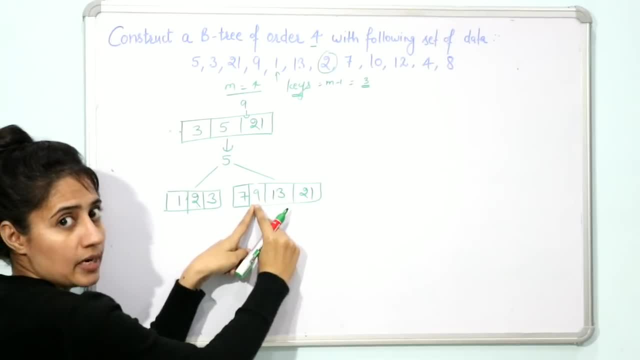 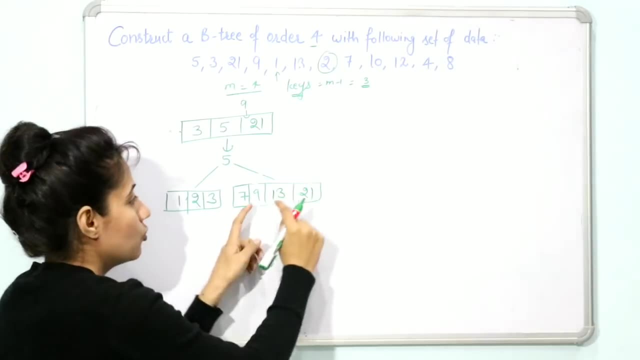 So here 9 would be middle element, So where 9 will go To its This node's parent And you can say one level up. So where should 9 go Here? 5, And we can insert 9 at this place Because we cannot have maximum key. 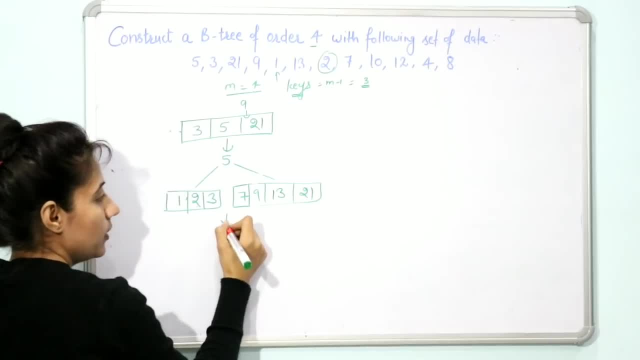 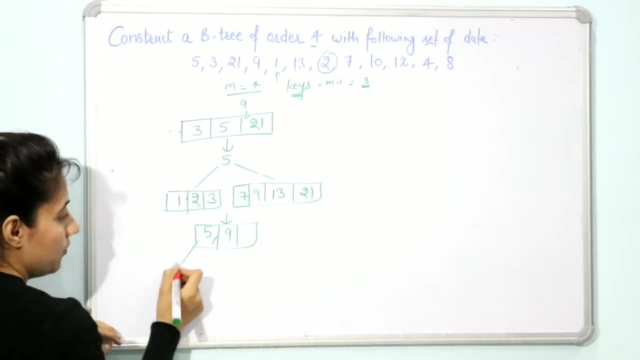 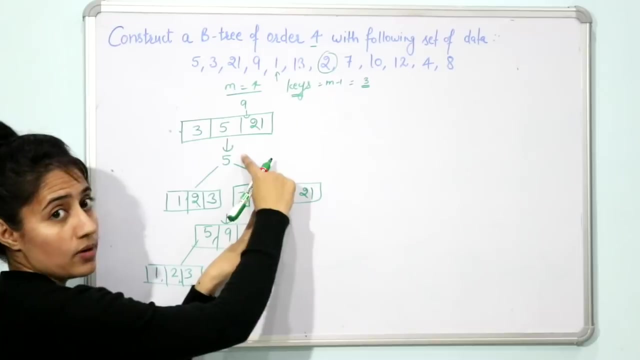 3 and we have only one key. Now the tree would be 5 and 9. Left part of 5 is 1,, 2 and 3, See 9. if one level up Means, this node would be split in 2 parts, So 9. 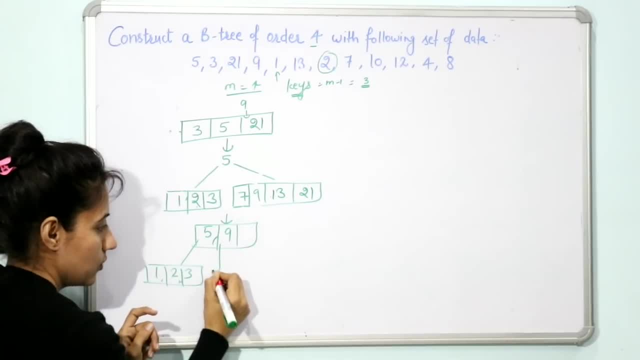 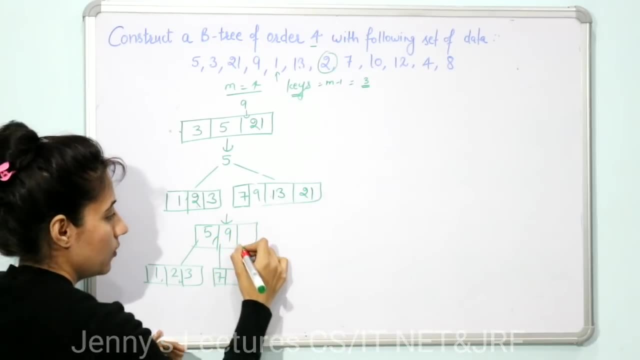 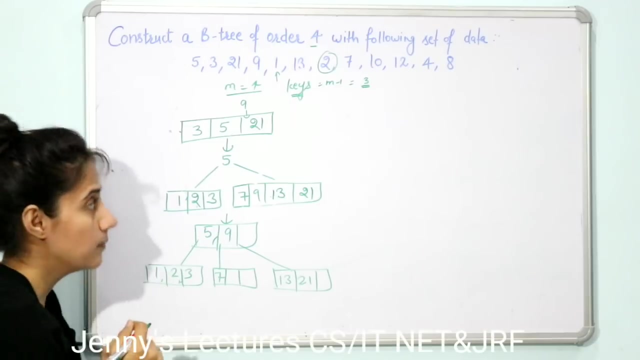 So 9's left child would be 7- This one 7 is here- And 9's right child would be 13 and 21 Here. what will go? 13 and 21, Fine. Next is 7. we have inserted. Next element is 10. 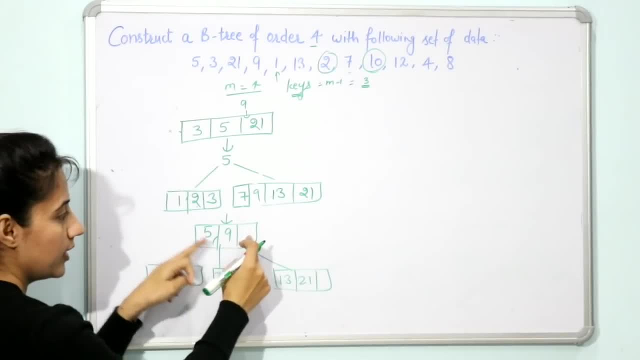 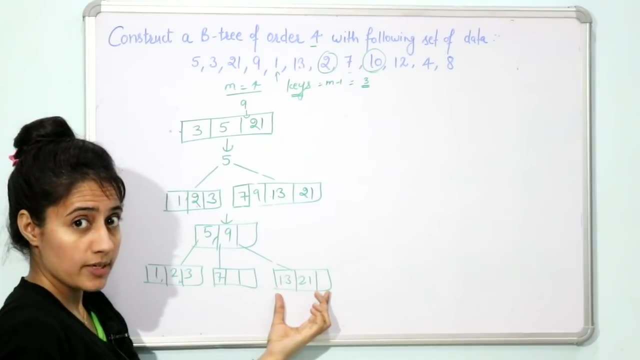 Now compare 10 with 5 and 9. If 10 is bigger than 5 and 9- So it would go to the right part of 9- Then 10 can be inserted here. Now find out 10's proper place. 10 is less than 13. 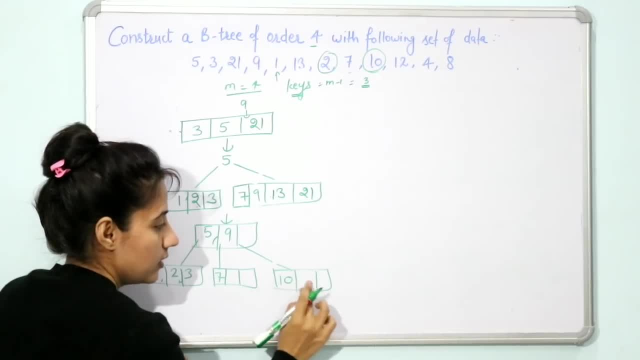 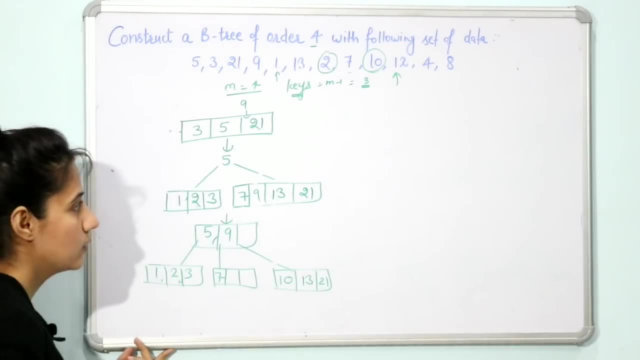 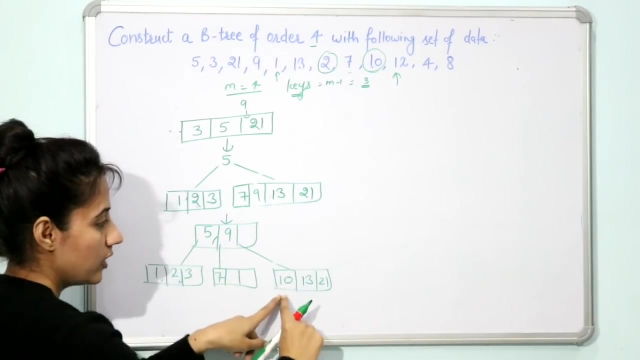 So 10 will be inserted here, 10. After that here is 13, And here will go 21. Fine, Next is 12. Now find out proper position for 12. 12 is also greater than this 9, So we will go to the right part, 12. 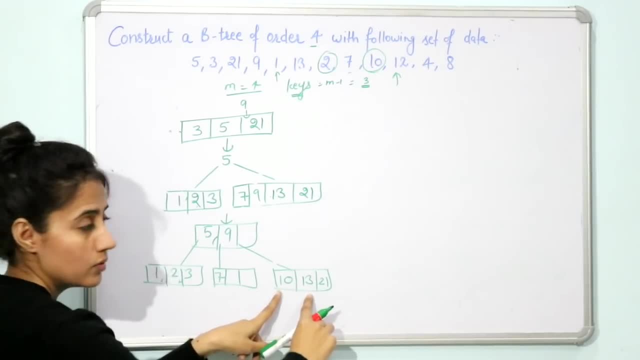 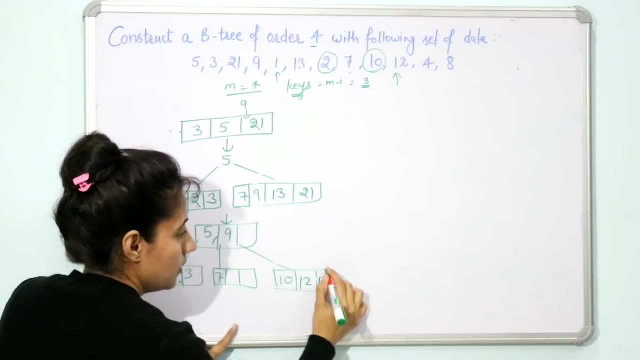 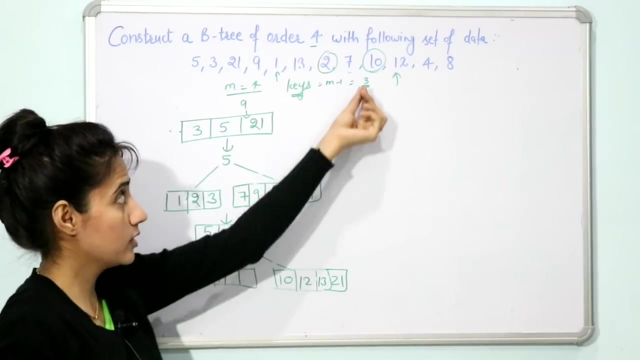 Where can it be inserted here? after 10 and before 13? So where should 12 be At this place? 12, 13 Into 21. It should be here, But you cannot insert this at this place. Why so? Because maximum keys can be 3. 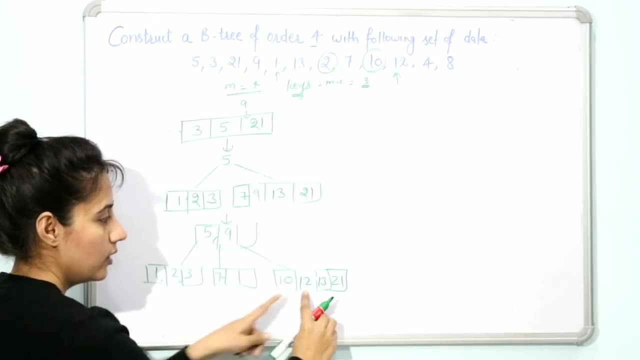 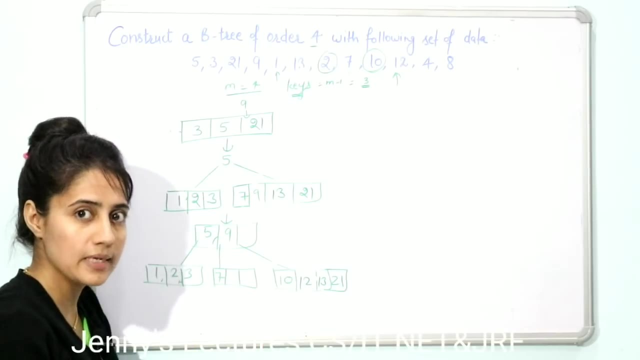 So splitting would be done. Where will be splitting? Middle element? What will be middle element? 12? Left biased tree can take 12 or 13, But we are working on left biased, So we will consider 12 as the middle element today. Okay, That middle part. 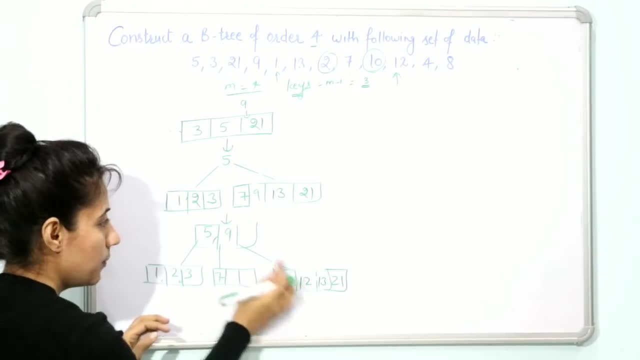 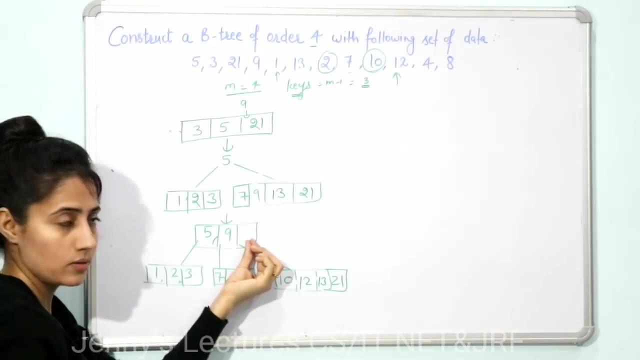 Middle element would go one level up. We can say to its parent node: Its parent node is 5 for 9, This node. So where will 12 go To this? We can insert 12 here, Because one place still we have left. Now the tree would be. 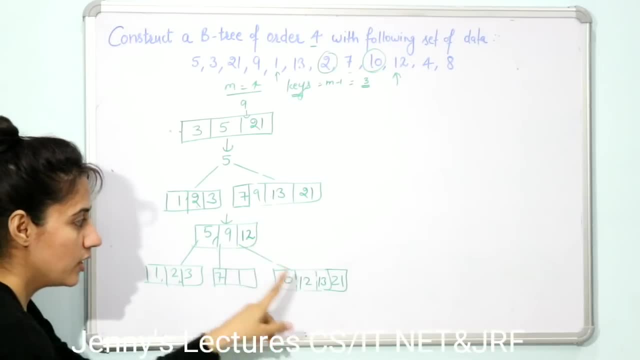 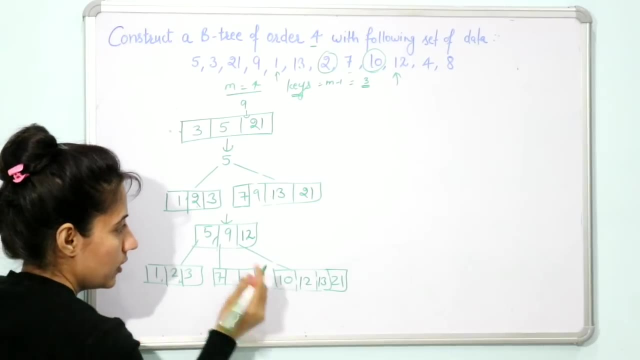 I am updating in this. 12 will go here, 12 will go up. Then this node would be split in two parts. 10 would be the left child of 12. Okay, What will be left in left of 12? Only 10. And What will go in right part of 12?? 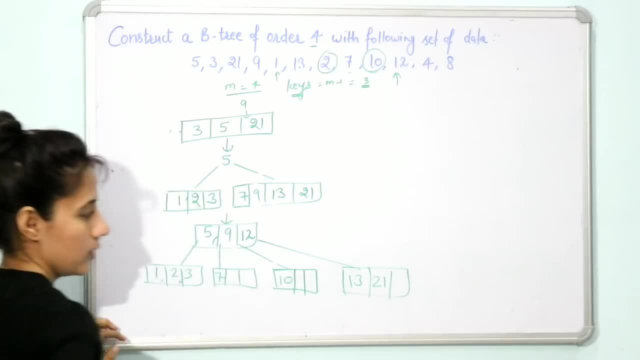 13 and 21. Okay, Right part of 12. Now next is 4. Don't compare: 4 is less than 5, So we will go to the left part of 5. You have to insert 4 here. Where can you insert 4?? 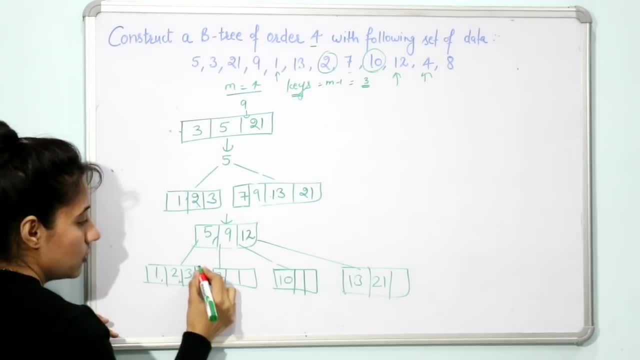 1,2,3 after 3. Where should you insert 4?? It should be here, Okay, But we cannot insert it Because Obviously maximum can be 3, So Splitting would be done. What will happen in splitting Middle element? What will we consider as middle element? 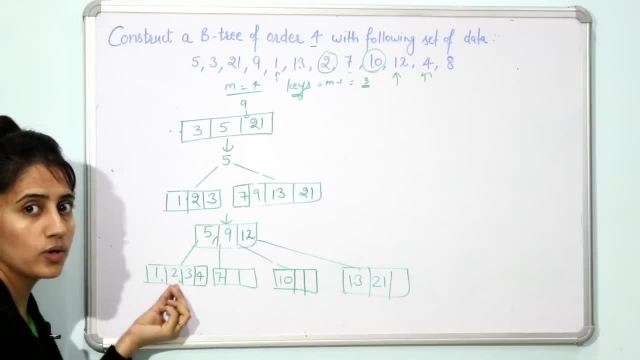 2, Then 2 would go 1 level Upper. you can say to its parent: node, See, If You have 2, 2 will go at this place. If 2 will go up, Then 2 is obviously less than 5, So it should be inserted here. 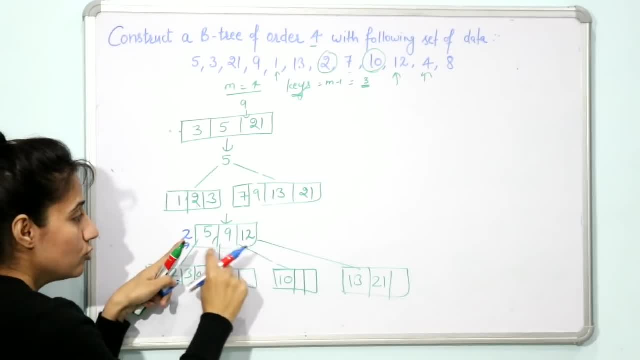 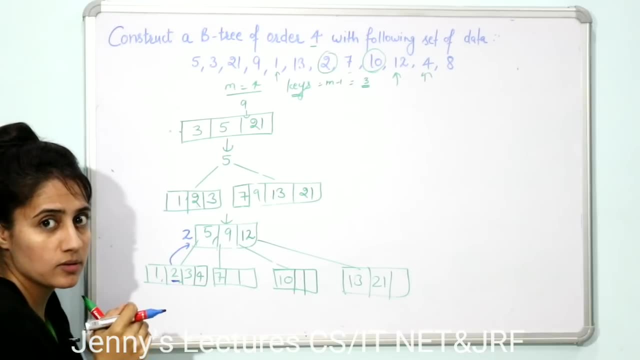 2,5,9 and 12, But Here also we have: This node is also full, Because 3 is already there, So we cannot put 2 at this place. So here also again, what will happen? Splitting will happen Until we find out the proper position. 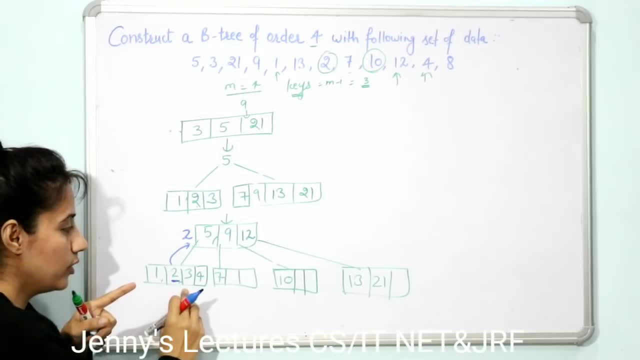 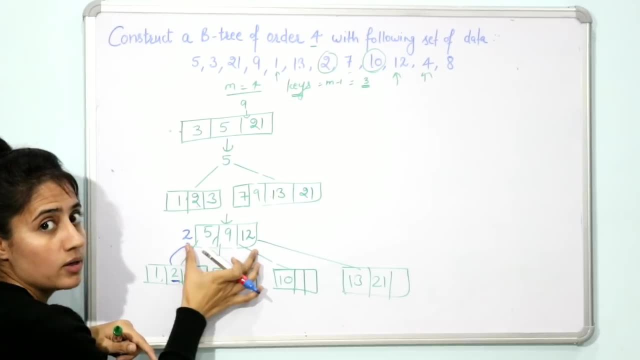 So splitting will keep happening again and again. Here splitting happened, 2 went up. If it goes here, In that case here also splitting will happen And this part will split What will happen. The middle element will go 1 level Up to its parent node If there is no parent. 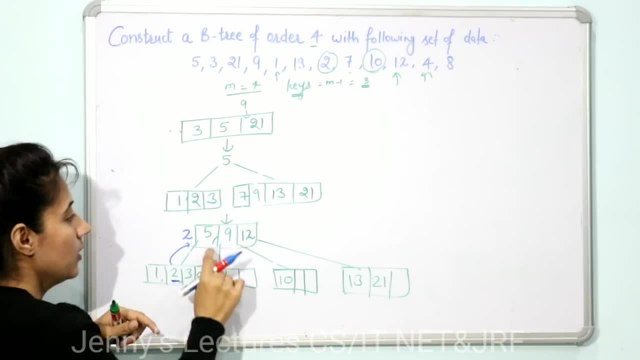 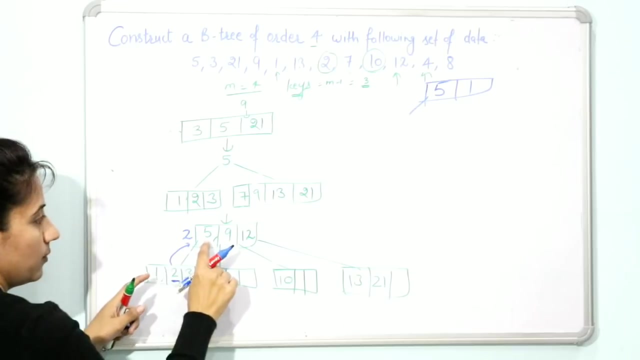 Then the middle element would become the root of this tree. Now, This middle element, We will consider this 5, Because The tree is left biased, So The tree would be 5. 5 went up, This node would be splitted. Now What is the left part of 5?? 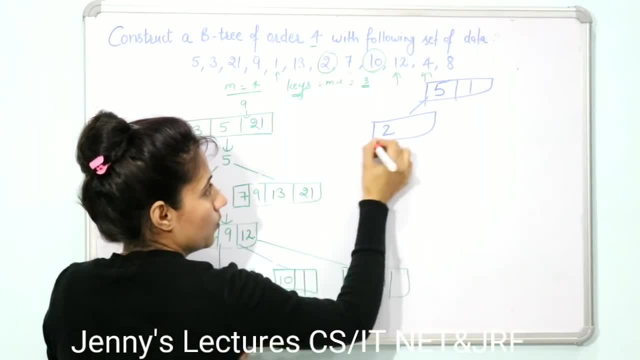 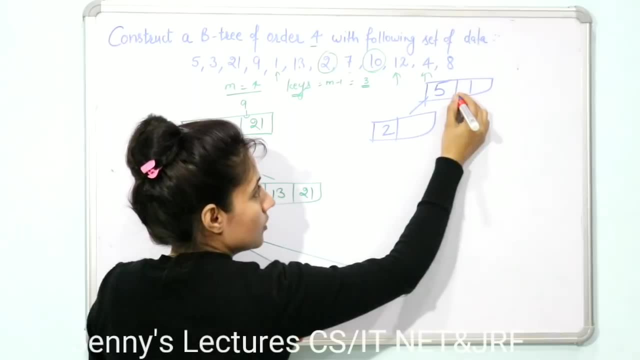 This 2, Fine, And what is the right part of this 5? Right, children, 9 and This 5, 9 and 12. Now come to this level. Now, what will be the left part of 2?? What will be the left part of 2?? 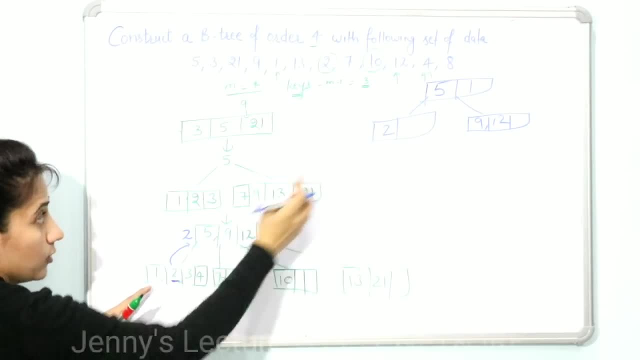 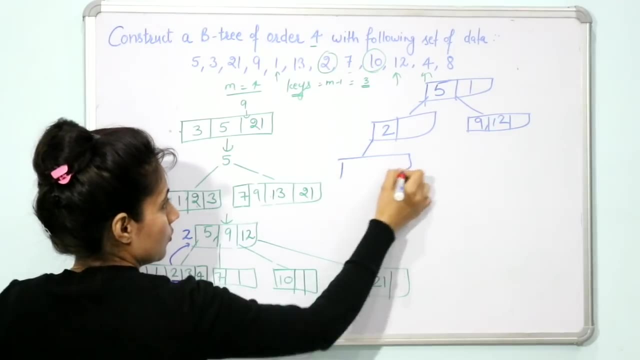 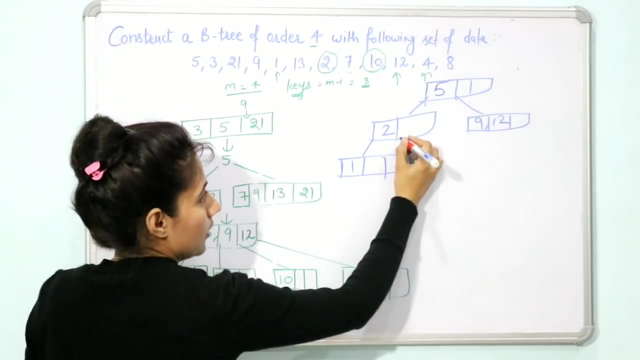 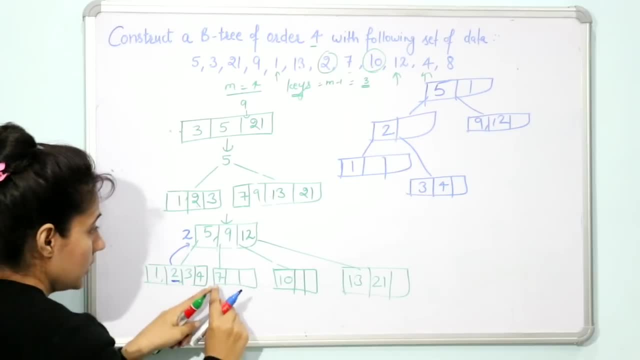 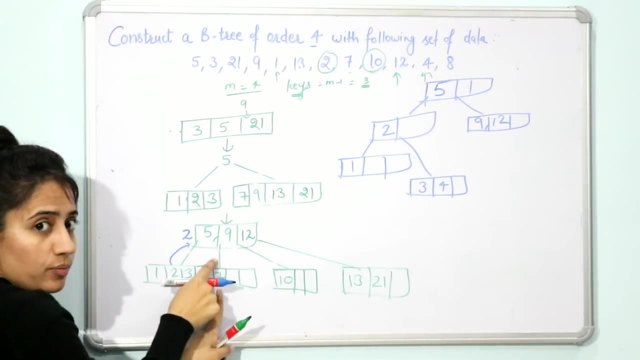 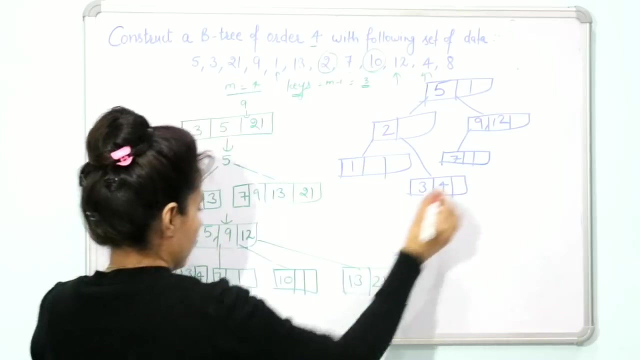 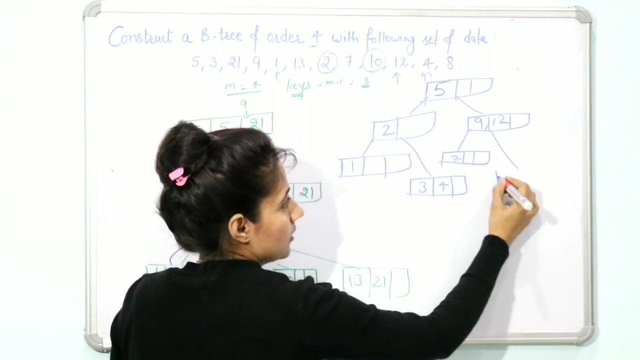 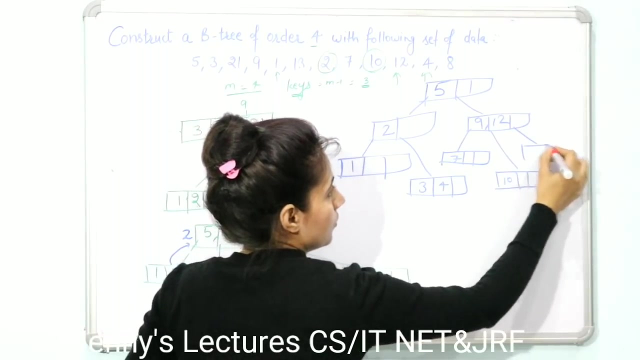 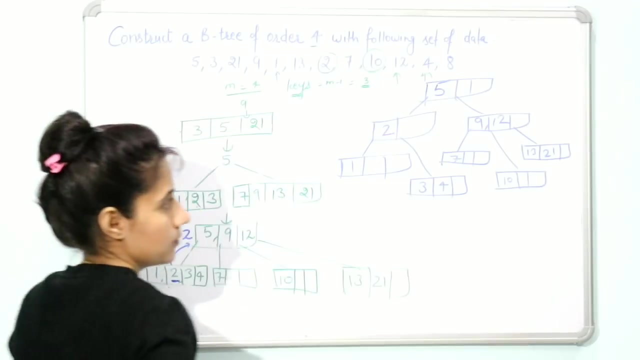 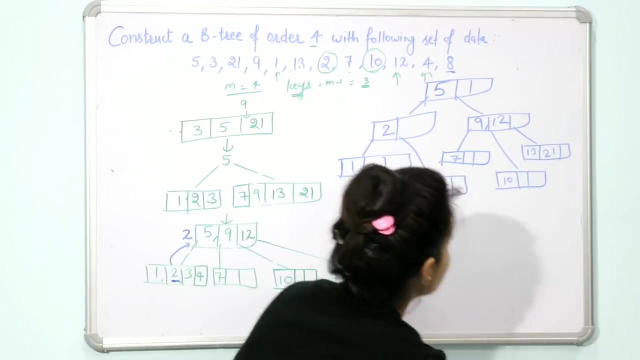 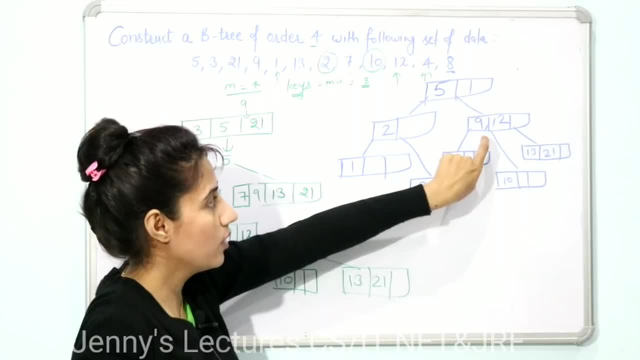 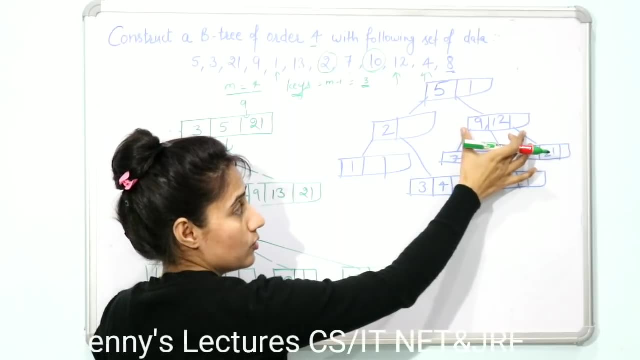 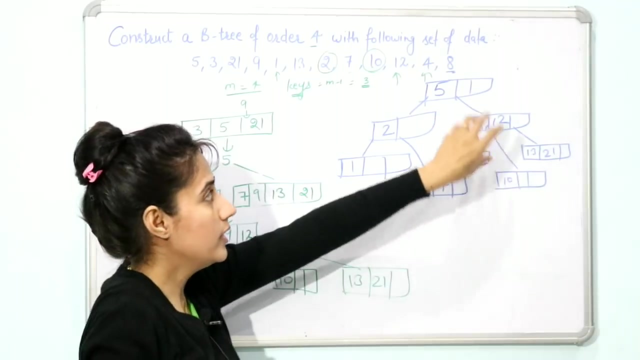 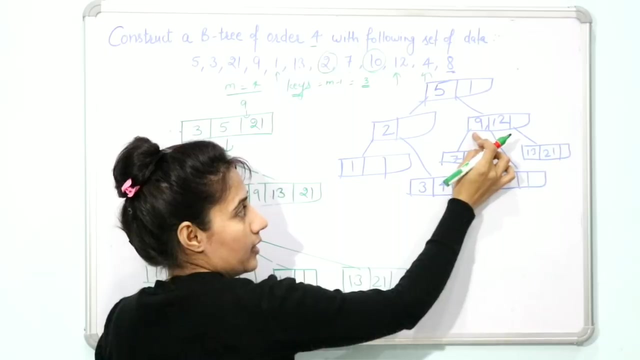 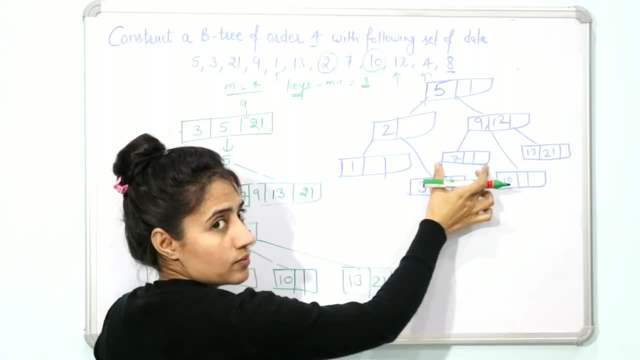 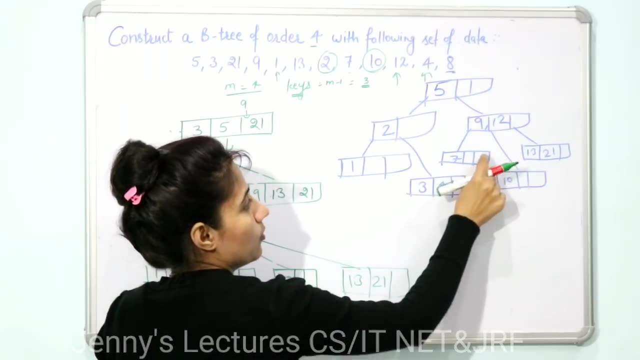 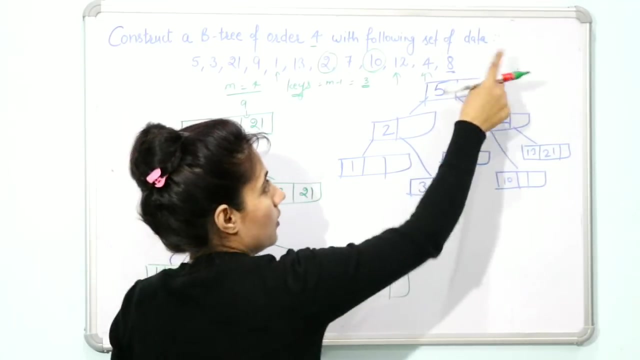 okay, see now this node is leaf node. fine. this is our 7 leaf node. below this there is no left or right part. now find out the proper position for 8. 8 is greater than 7, so where your 8 got inserted at this place, fine. next, we don't have. so this is the final b tree of order four. 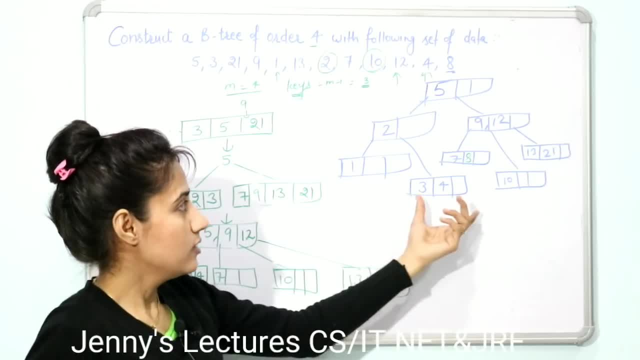 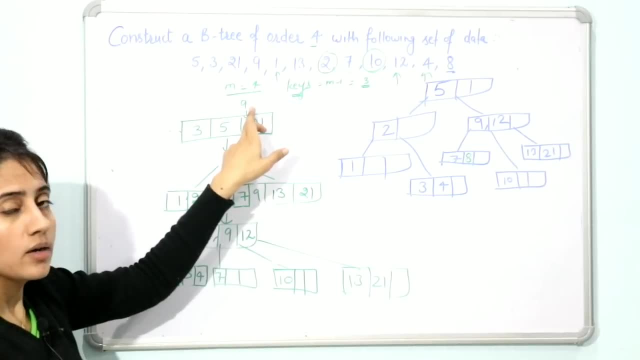 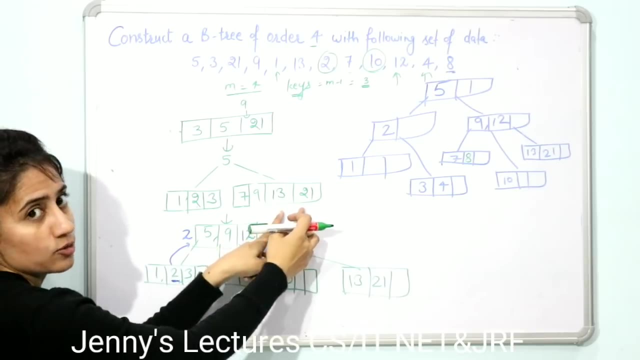 fine. another variant is say: this is also right. another variant is that right biased tree, you can take this 9 as a you know middle part and you can put 9 at this place, 35 at this place and 21 at this place, this place. like this you will proceed and that one another tree would be there. 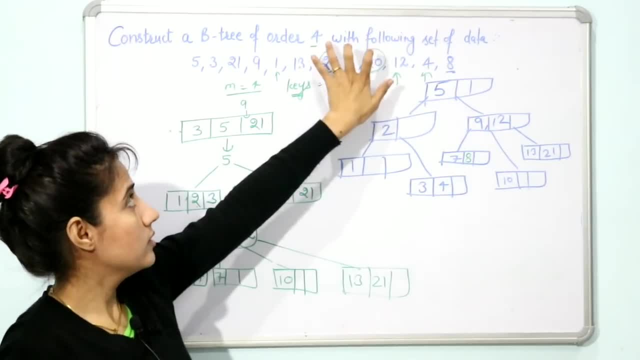 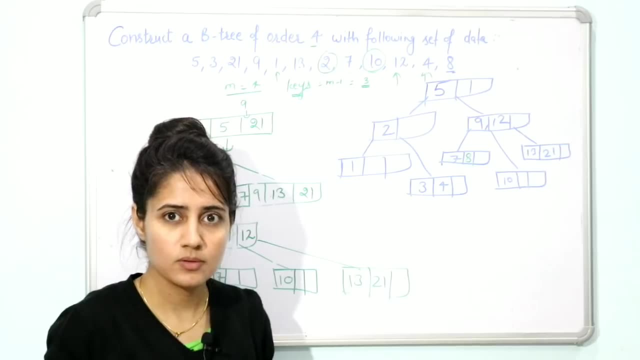 though job apka even number, hotel. that order is given with this even number to up get two trees possible. heaven is left biased and one is right biased, fine, so I'll see you in the next video. I still then bye, bye.